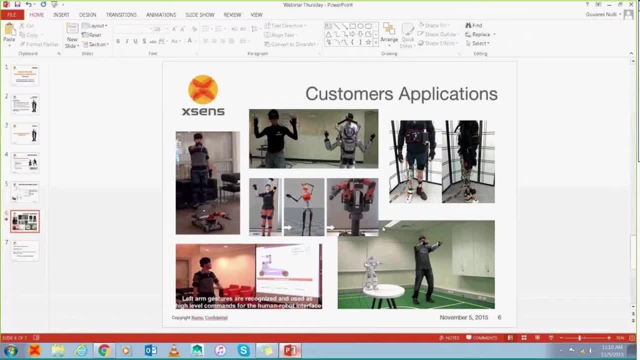 before we pass things off, are a few customer applications that have been done in the human-robot interaction field using our MVN Biomix product. The two examples that you see on the left, here and here, were done by a customer using the MVN Biomix. 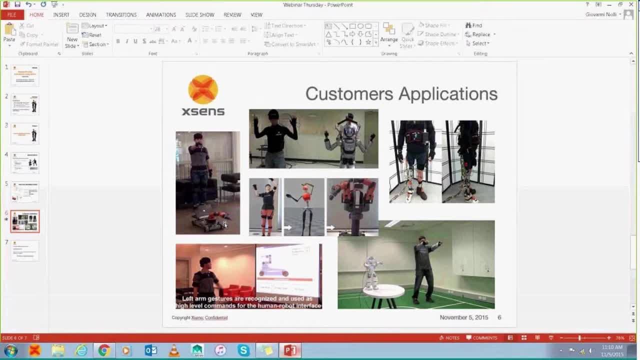 to control movements of a robot based on specific movements of the body. A movement of the arm could easily move the robot forward or backward, allow a turn or allow changing in the software. In the center and in the lower right you see applications where direct movement of the human body. 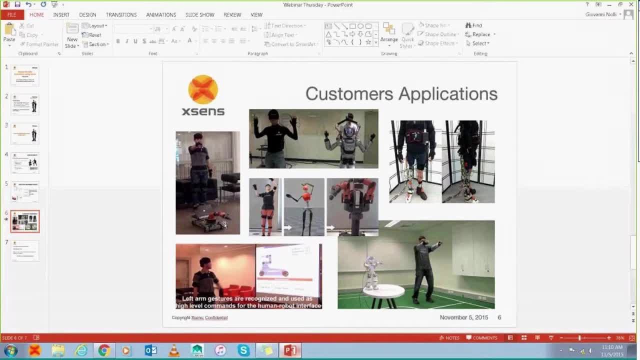 is mapped to a humanoid robot. These applications are quite easy to use because it allows full-body movement to control exactly what a robot would be doing as well. The last application in the top right corner is an integration of the MVN Biomix system with a type of robotic application. that seems a little bit different. 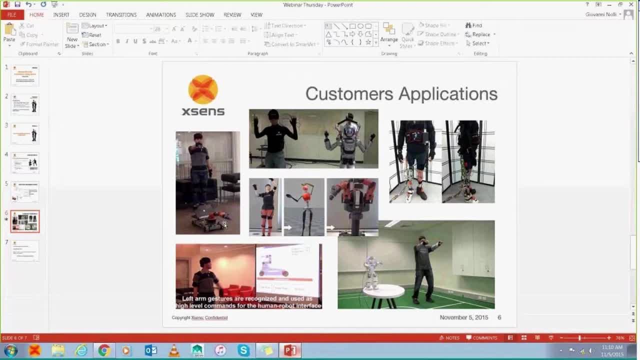 This is the use of a power prosthetic where the sensors are placed on the body, placed directly onto the prosthesis, to measure how the prosthesis is moving along with the human body. All these types of applications are made possible with our MVN Biomix product. 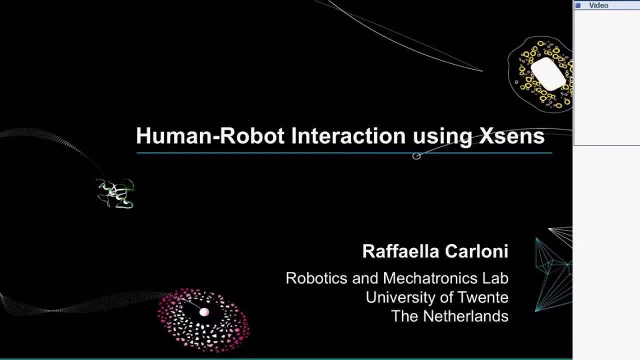 In these 15 minutes, I'd like to tell you a little bit about the terrific opportunities for applying the technology developed by XSense, And I'm going to show you some results that my research group at the University of Trent in the Netherlands has obtained within the Project SharePoint. 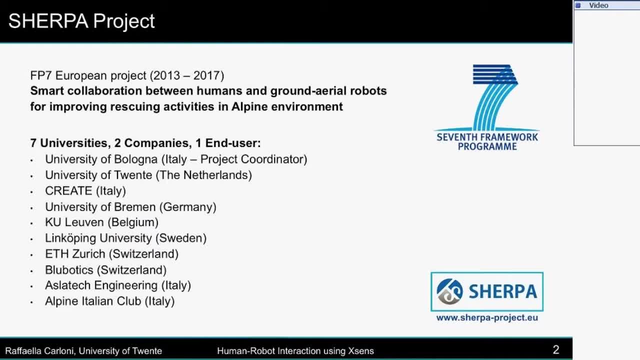 So I will briefly introduce the SHERPA project. It's a project funded by the European community within the 7th Framework Program And SHERPA is an acronym and it stands for Smart Collaboration between Humans and Ground Area. Robots for Improving Resting Activities in Alpine Environments. 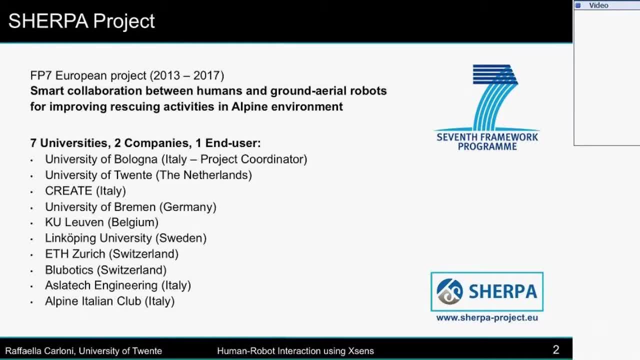 It is a big project with a consortium of 10 partners, among which there are 7 universities in Europe, two companies and one end user, the Alpine Italian Club, which is actually providing us with the problems that our robotic system has to be solved. 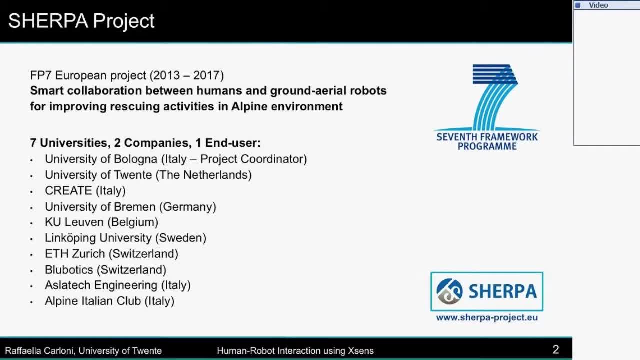 So this Alpine Italian Club is a non-profit, non-political organization devoted to search and rescue operations in mountains and caves. It has 7,000 volunteers with more than 6,000 operations per year. So already when we were writing this project proposal, 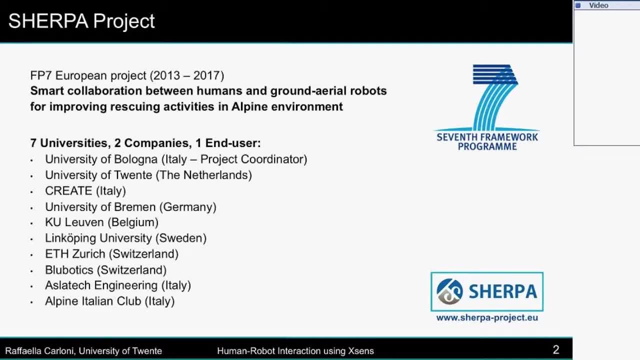 XSense entered in the advisory board and the University of Trent here in the Netherlands and the consortium created in Italy, University of Federico Secondo, indeed, in Italy and University of Bremen in Germany. we are using XSense and VN Biomech. 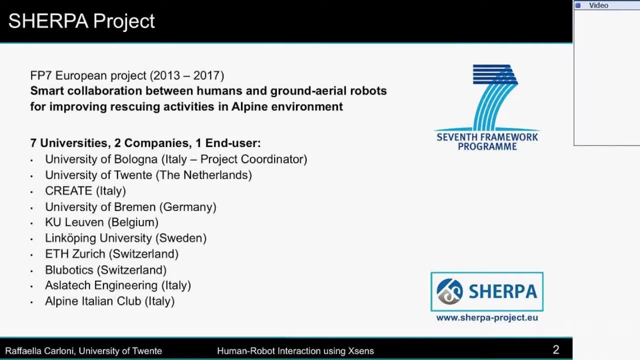 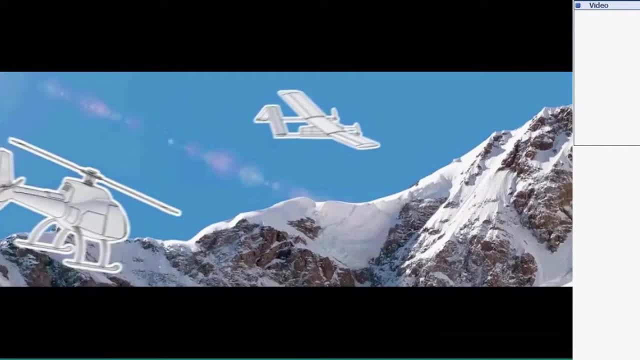 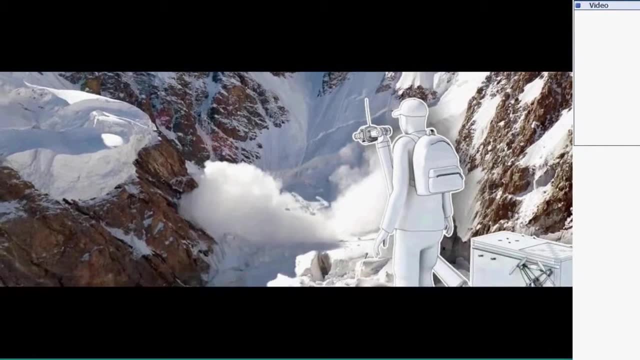 So just to give you a better idea of what the SHERPA project is, what the SHERPA project is about, I'm showing you this clip. So you see mountains, a winter scenario, you see flying vehicles and here you see also a human rescuer. 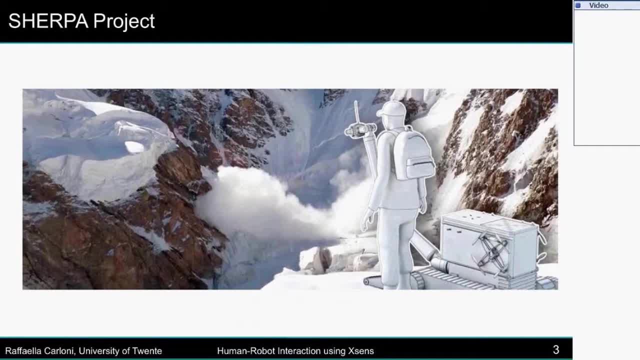 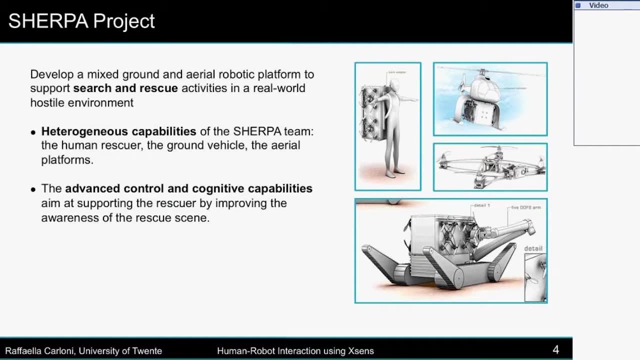 close to whom there is a rover endowed with a robotic arm. So the goal of the SHERPA project is to develop a platform which is mixed so ground robots and aerial robots, which should perform, together with the human rescuer, search and rescue activities. 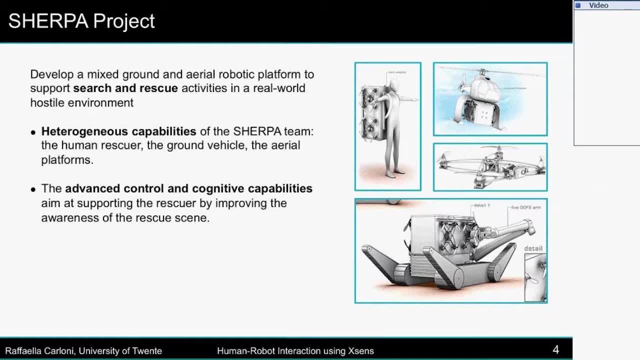 in real-world hostile environments such as the one that I showed you in the clip. So we have a SHERPA team which is composed by different actors and they have heterogeneous capabilities, So the human rescuer is very busy in the search and rescue activity. 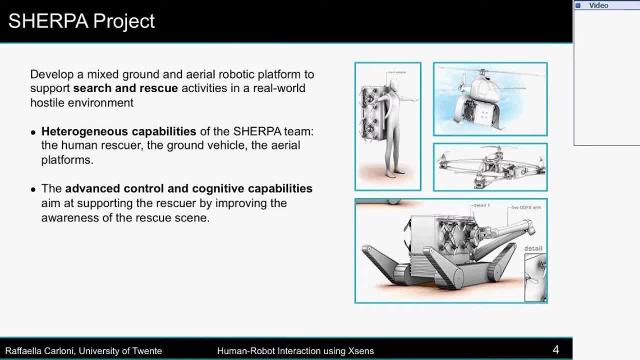 and he has higher cognitive capabilities. And then there are robots which are implementing autonomous behavior. but we want the whole system, so the robot and the human, to work together with advanced control and cognitive capabilities, so that the rescuer is supporting and his awareness of the rescue scene. 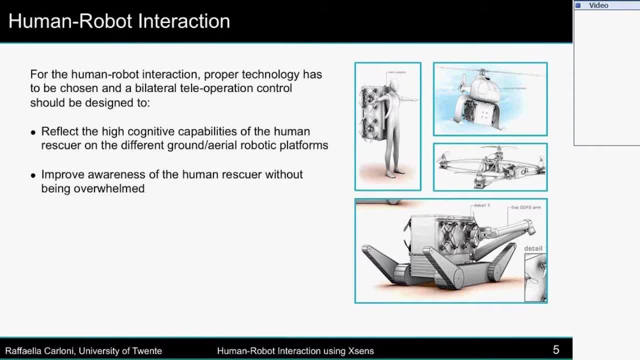 is improved Here at the University of Pente. besides developing the robotic arm that is mounted on the rover, we are focusing on human-robot interaction, And for that we needed to select the proper technologies and also to develop bilateral teleoperation control. 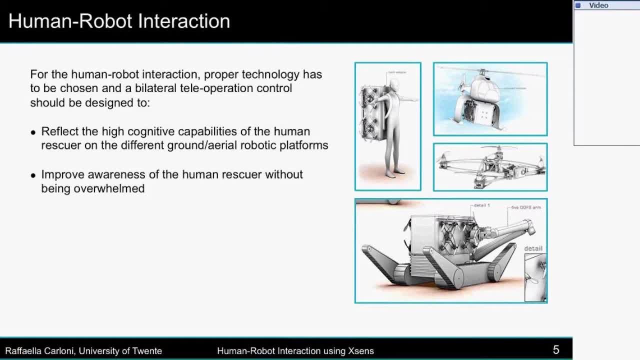 So what does it mean? As I said, the human operator is busy and the robots have an autonomous behavior to support the human activity By sketchy gestures. the human rescuer should instruct the robots in order to properly tune and overrule the autonomous controller. 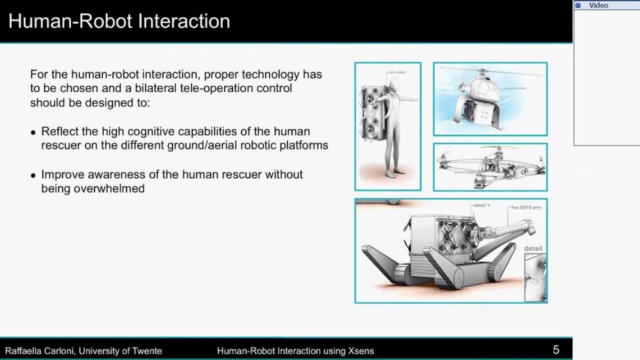 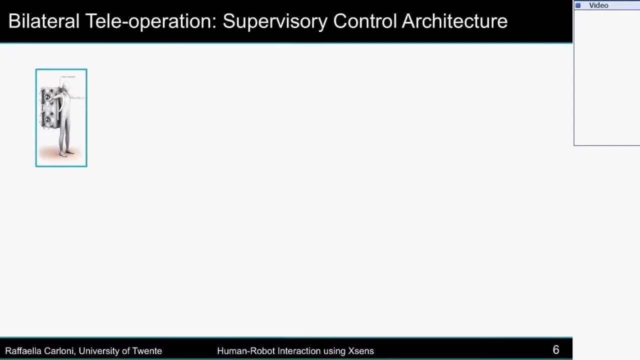 and also the human rescuer should receive back information, And the information that the human receives back should not overwhelm him or her. So here, as I said in Pente, we have developed a bilateral teleoperation scheme. We call it Supervisory Control Architecture. 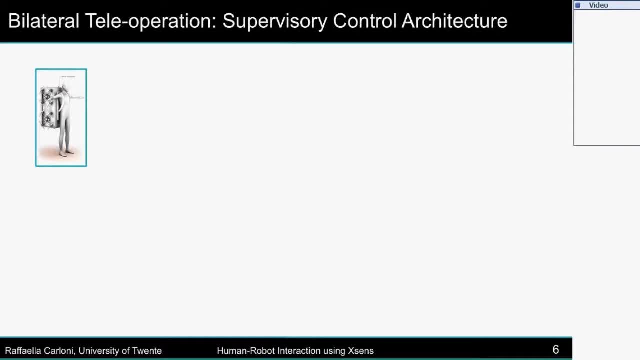 So, if we are focusing on the bilateral teleoperation of the flying vehicle, we have the human rescuer, we have a drone, so the flying vehicle that should scan a certain area and we need to realize this communication and then we can make it bilateral. 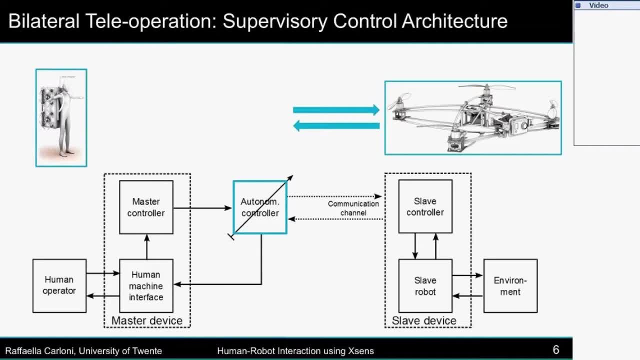 So from the human to the drone and vice versa. So here in these blocks, you see the seven blocks typical of any bilateral teleoperation. So from left to right you see the human operator, then there is the master device, which basically consists: 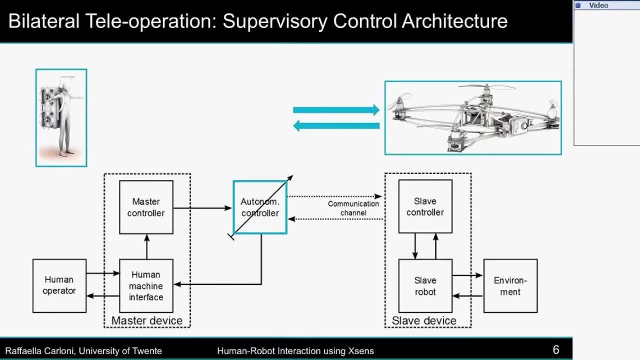 of the human-machine interface and its controller And, as we are seeing it, this master controller gives some information to the autonomous controller of the slave And in this case, the slave is the drone which you see in the right part of this block scheme. 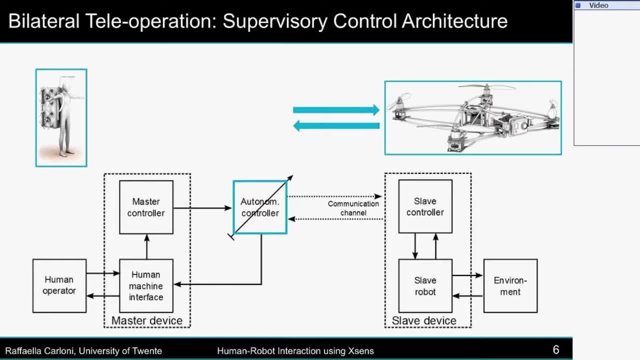 The slave might or might not interact with the environment, And the communication between the master and the slave is done through a proper communication channel. So I'm going to give you some details about the autonomous controller, And before that I want to point out that 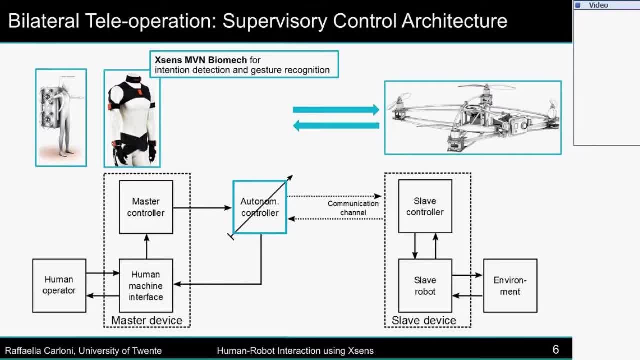 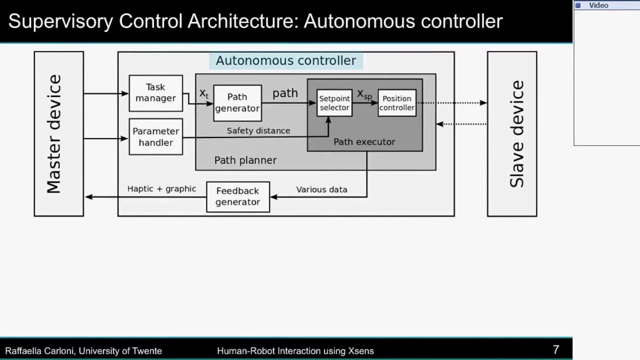 for the human-machine interface part, we have selected the XS-MBN Biomech for intention detection and gesture recognition And I'm going to give you some more details now about while I'm entering in the details of the autonomous controller. So we have the master device on one side. 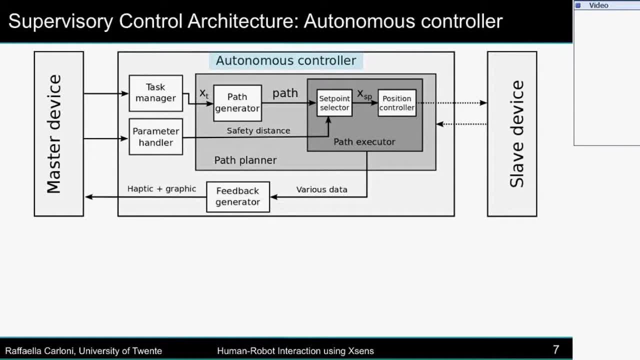 and the slave device on the other side. So the human interface is on the master side, of course, And through the task manager and the parameter handler, we are actually interpreting signals that are coming from the human. So the task manager, for example, 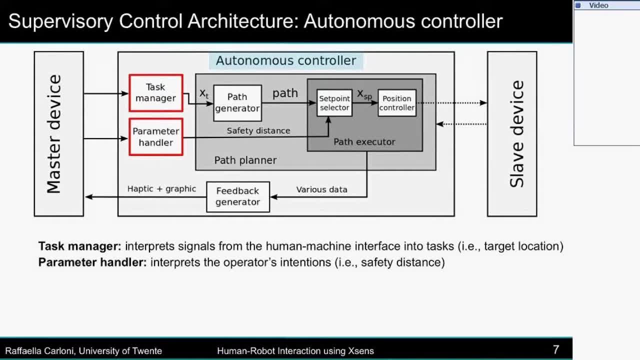 is interpreting the signals from the human-machine interface, so the X- and suit into task like, for example, deciding about the target location. So XC here says for the position that the flying vehicle should reach. Then there is this parameter handler here. 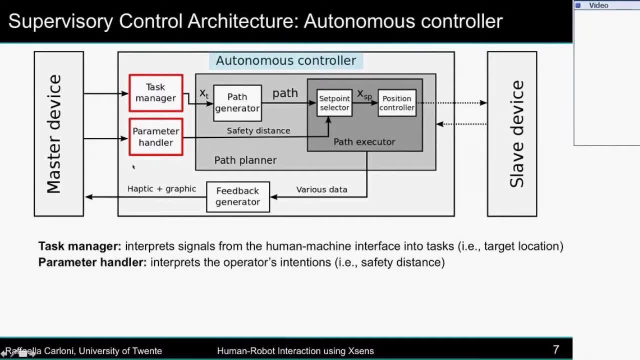 This block interprets the operator's intention. So, for example, if we are assuming that the autonomous controller has a safety distance, meaning a distance that the drone has to keep from obstacles, actually the human operator can influence the safety distance because in the autonomous behavior, 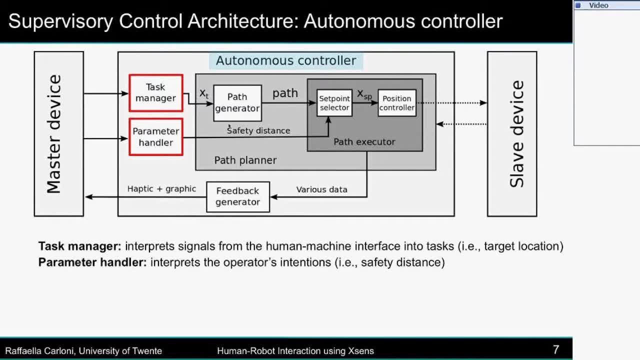 the drone should play safe, and so this safety distance might be big, But the human operator, since he or she has a higher cognitive capability, can overrule this safety distance and, for example, make it smaller. Then once, safety distance and the final target position. 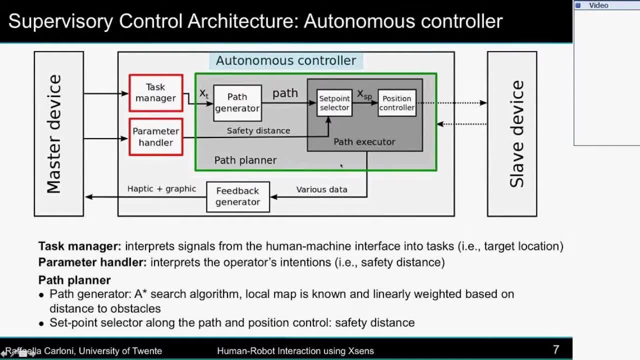 has been selected. there is this other block, which is the path planner, So we have the path generator and the path executor And, of course, there will be a position control, a low-level control on the drone And here in the bottom part. 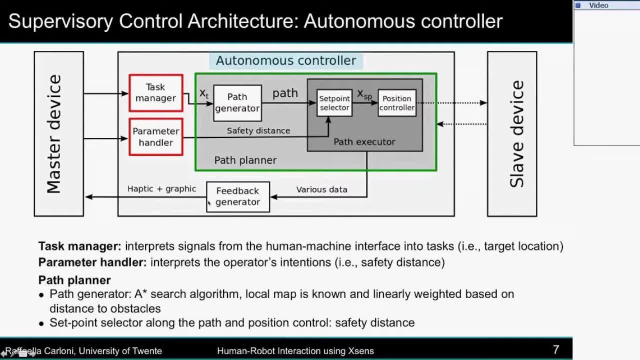 of this figure. here there is the feedback generator, So the human operator will receive back some feedback in terms of haptic feedback and graphic feedback from the slave side, back, indeed, to the operator. So for the path execution part, I want to show you: 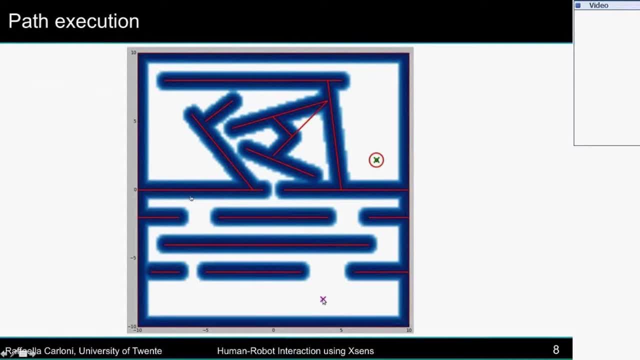 the autonomous behavior of the system. So here we have this red circle, We have the starting position of the drone And here, where there is this X, purple X, it's the target position. So the red lines are obstacles and the blue shadows 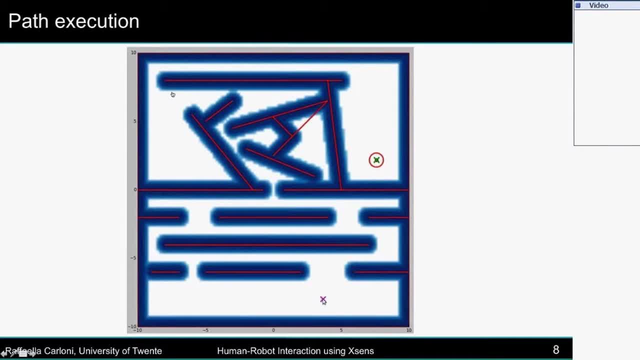 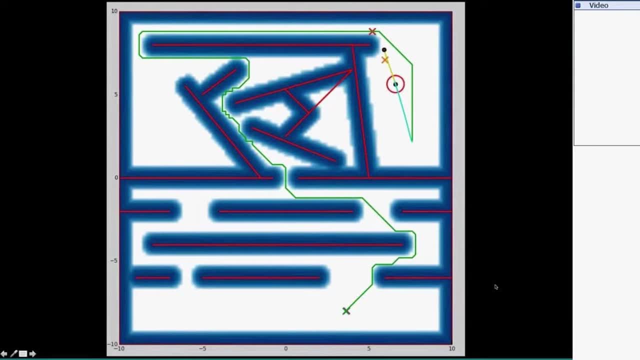 are the safety distance that the vehicle should keep from the obstacles. So when the algorithm starts, we select the target, which is indicated by recognition of the human gestures through the X and suit, And then, once that target is selected, there is a path generation. 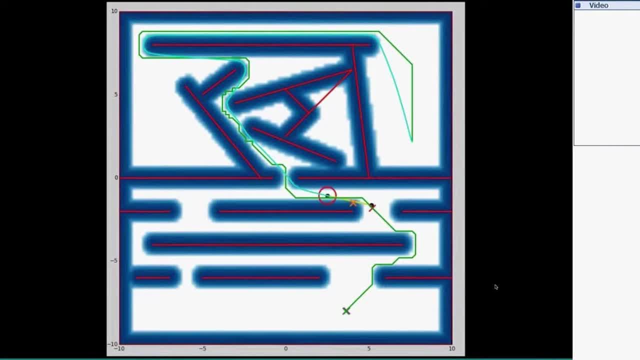 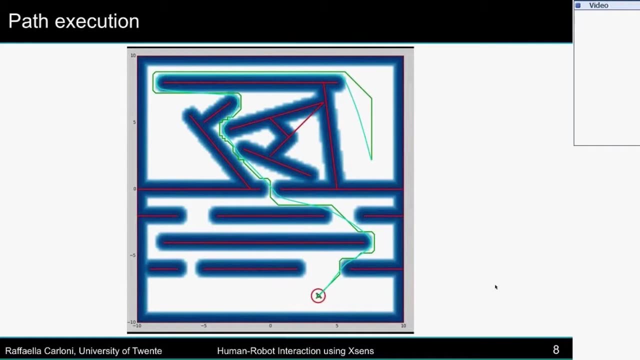 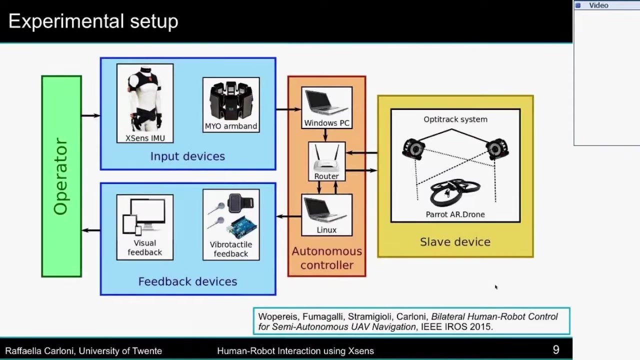 and then the UAV will autonomously go towards the target. But the human operator can overrule the information about the safety distance. So we are using again the X and suit in order to change and maybe to reduce the safety distance. So before showing you, 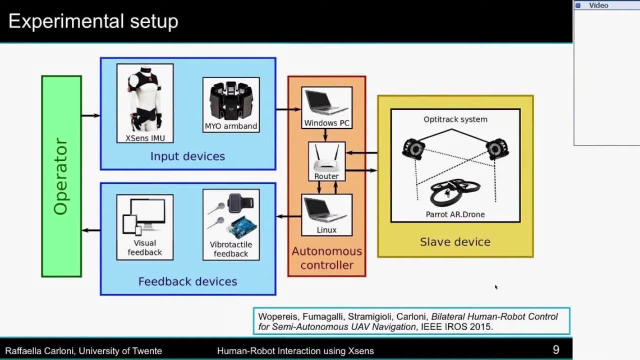 the video of the experiments. I want to spend a few words about the complete software architecture. So there is a human operator and the gestures of the human operator are read through input devices. So we are actually fusing different information from the X and suit. 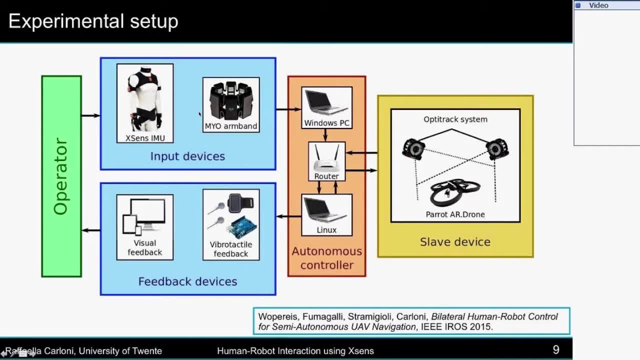 and the Mio armband, And those technologies are running on a Windows PC, which is here. Then there is the slave device and the autonomous controller is running on a Linux machine, And the communication in between those different Windows and Linux machines is happening through ROS nodes. 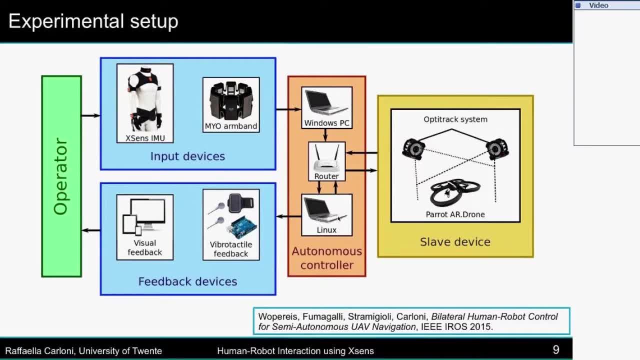 so the robotic operating system, So the X and suit, is publishing on the network information through an ODP channel with a frequency of 100. And those information are merged in order to realize and to influence and to overrule the autonomous controller, once the operator decides that. 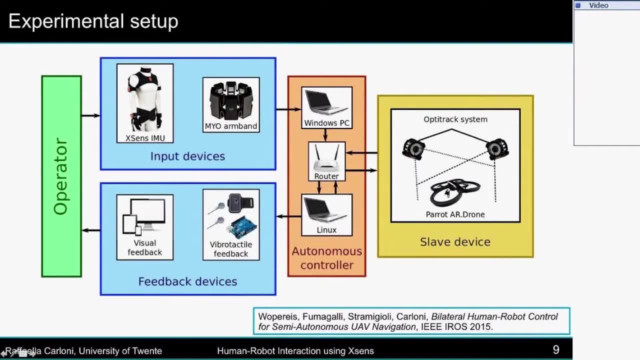 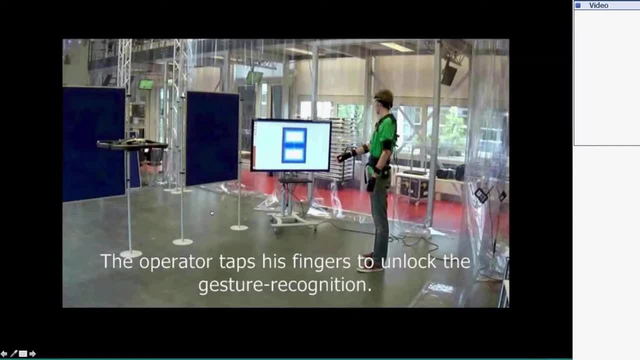 And of course, we have a feedback. So we have some vibrotactile feedback and we have a visual feedback. So I show you in this video which actually has been realized in our lab. So there is a human operator, There is a flying vehicle. 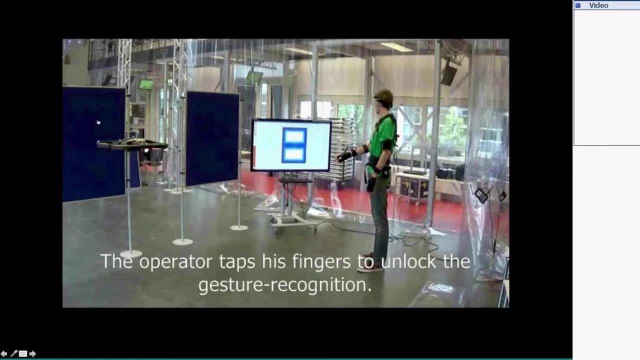 And then there are two blue walls here And there is a small opening. So the idea of this experiment is that the human operator will indicate a point behind the wall, But since this opening in between the two blue panels is too small, so it's below the safety distance. 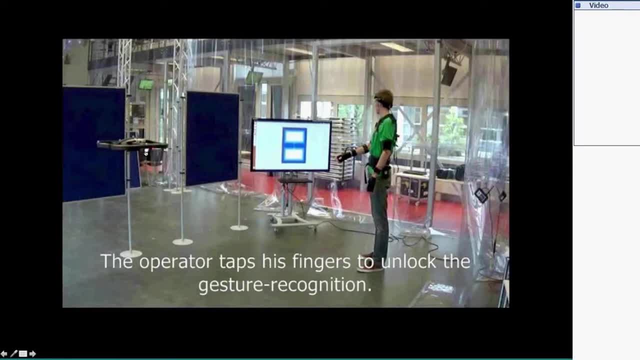 the flying vehicle will just stop in front of them. Then the human operator will overrule, by bending his arm, the autonomous controller. So basically, the drone will be able to reach the set point behind this blue wall. So the activation is done by tapping the finger. 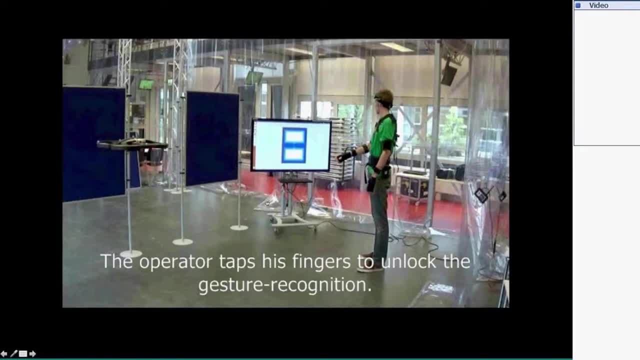 through the new arm band, while the accent suit is used to select the set point behind the panel. And also the safety distance is increased and decreased by bending the lower arm of the human operator. So I will show you the movie now. So the operator taps. 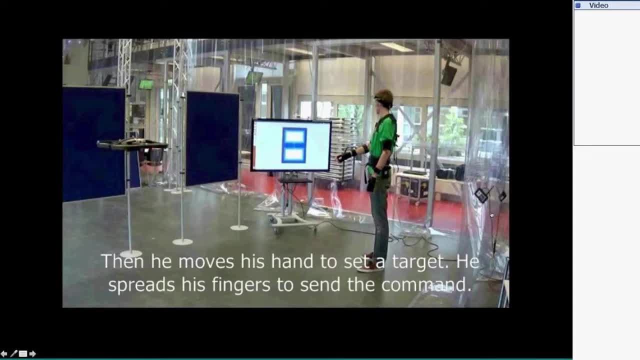 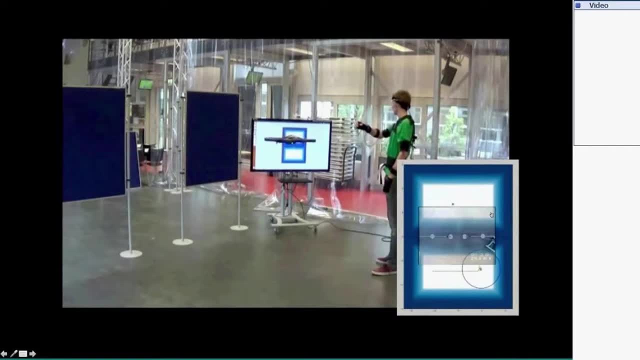 his fingers to unlock, Then he moves his hands to set the target. So you can see now that he taps the fingers- Initial position And then here it sets the new target, But the vehicle is just actually stopping because the opening is too small. 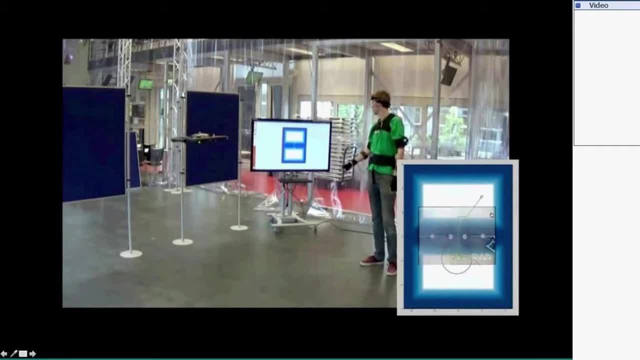 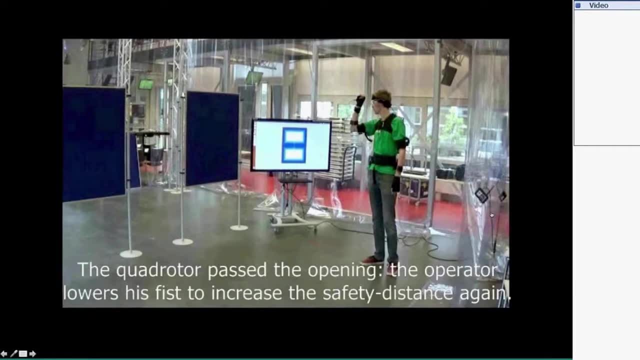 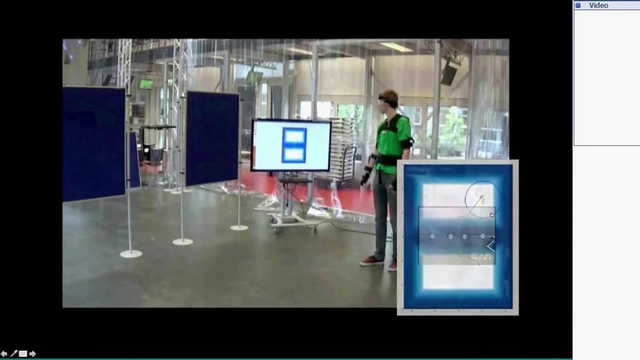 Then the human operator bends the arm, The safety distance decreases so that the vehicle is allowed to go through the opening, And then the human operator lowers the arms, The safety distance is increased. So here there is the top view, The blue circle is the safety distance. 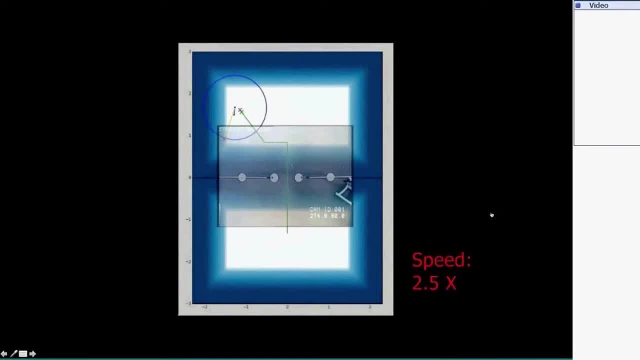 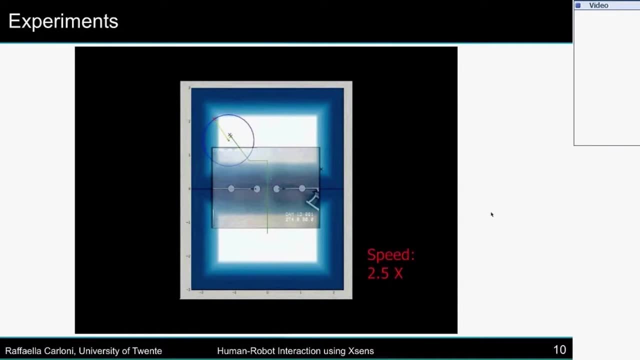 This is done in simulation: The safety distance decreases And then behind the wall, it increases again. So this is a bilateral tele-control, tele-operation controller with a supervisory control done by the human operator and by using the XN suit. Another example: 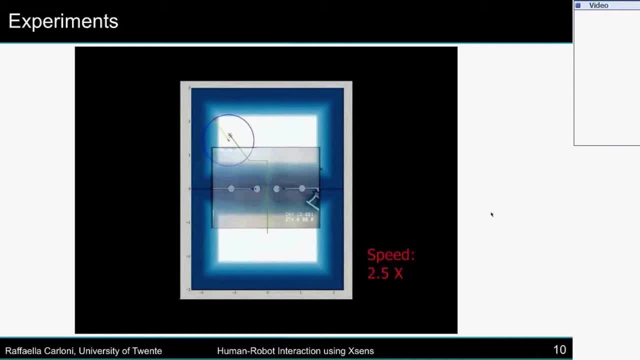 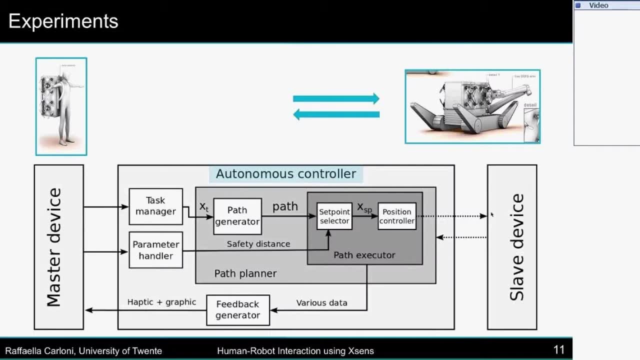 is the tele-operation of the robotic arm that is going to be mounted on the rover, And so the control architecture is very similar to the one that I presented. So there is the human operator, There is an arm, And then the controller is basically very similar. 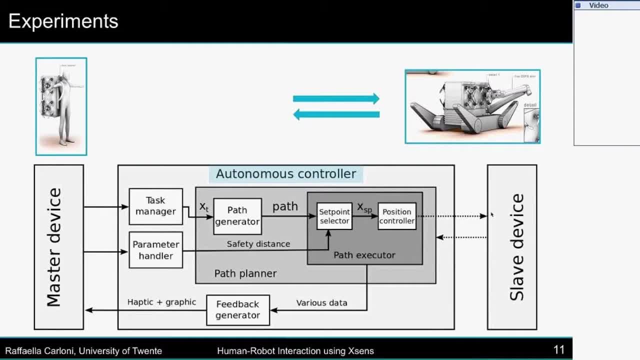 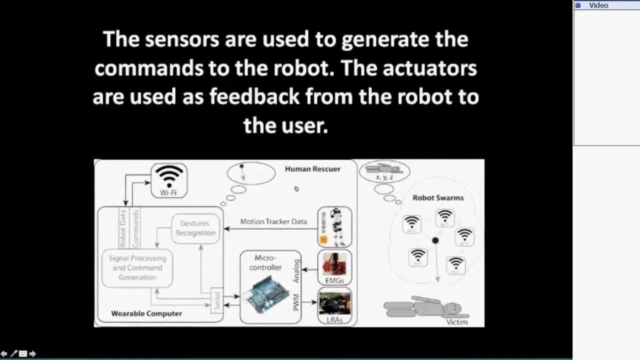 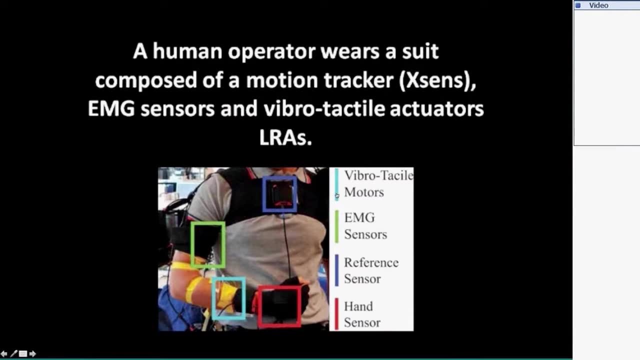 So I'll show you the one degrees of freedom case. So in this video- sorry, in this video you see, In this video you see again the human operator wearing the XN suit, And there are EMG sensors as well to detect the muscle activity. 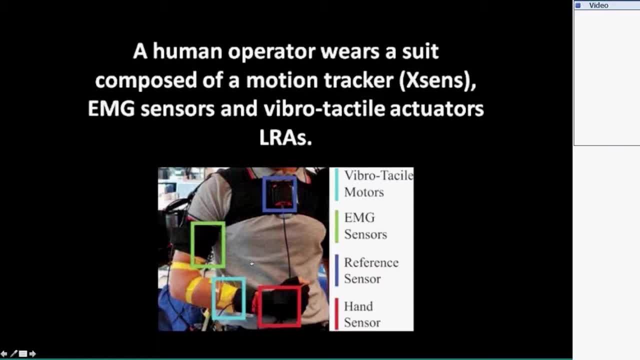 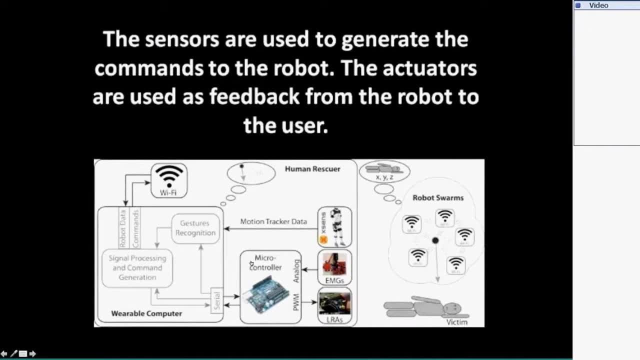 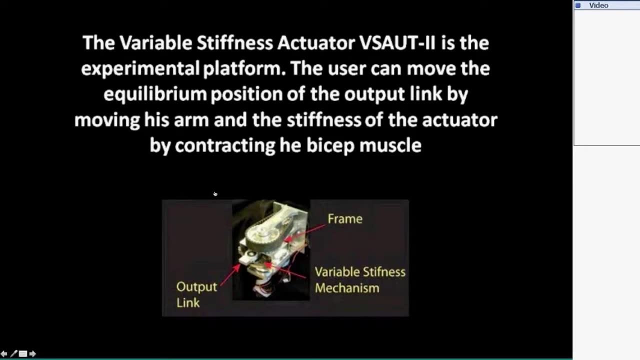 And then there are vibrotactile actuators in order to give feedback to the human operator. So the architecture is very similar to the one that we have just seen As an actuator system. so we are looking at one degrees of freedom. robotic arm. 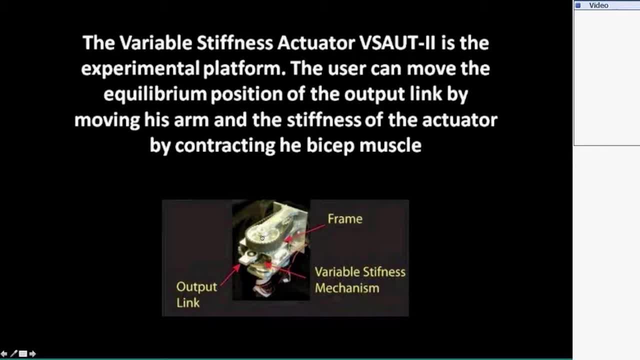 It's a variable stiffness actuator system So we are able to tune the output link, And that we are going to do by the motion detected of the human arm And then by using the EMG signals. we are using this variable stiffness mechanism. 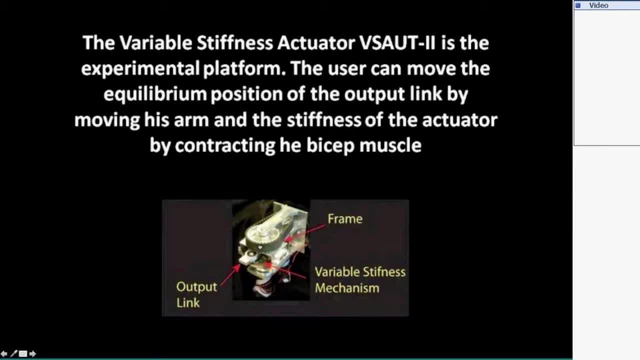 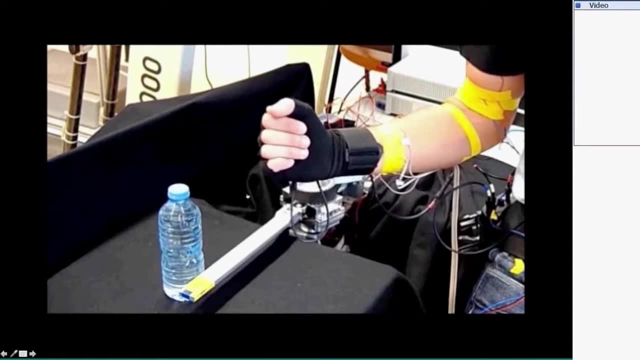 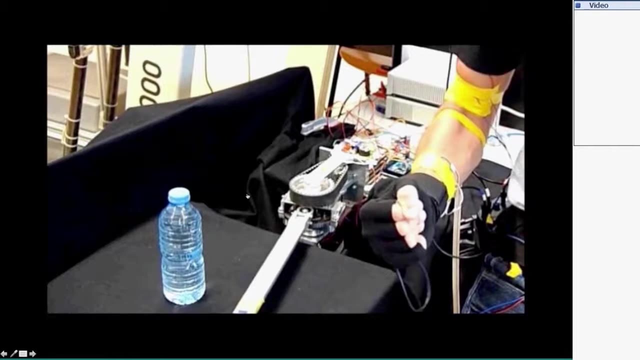 So basically, we are trying to reproduce the human arm behavior into the one degrees of freedom arm. So here you see that the motion of the human arm are reproduced through the reading of the XN suit to the motion of the robotic arm. While we are stiffening.